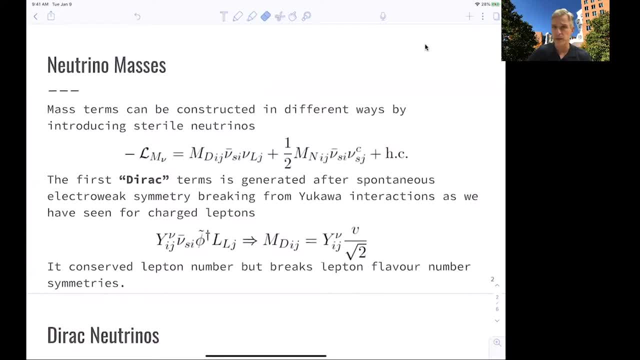 mass terms can be constructed by introducing so-called sterile neutrinos. The first way shown here in the Lagrangian is very familiar to you, where you have a left-handed component of a particle coupling via the Higgs boson to a right-handed component. Now, if we now 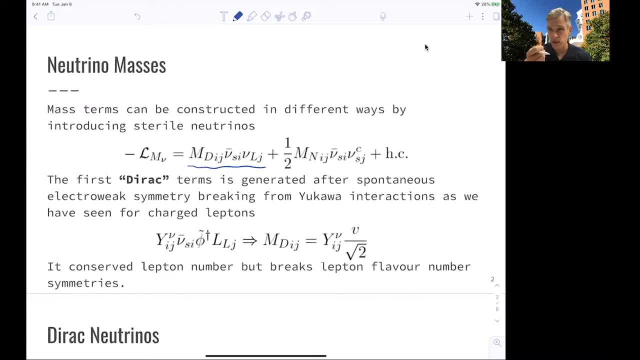 have a right-handed component or right-handed neutrino. that neutrino does not interact with a weak interaction and it doesn't interact with any other. Hence this neutrino, this right-handed particle, is a sterile neutrino, is not interacting. 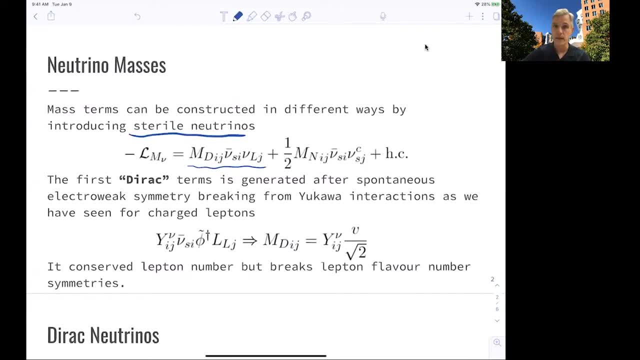 in any known ways other than with the Higgs field, with the rest of the standard model. The second way, the second mechanism, is using Majorana particles, particles which are their own antiparticles, And we'll look in How this is being implemented. 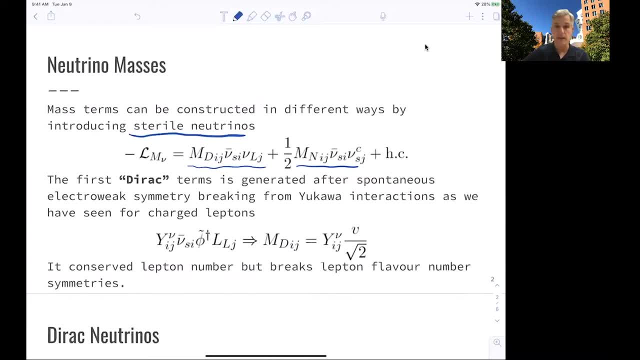 So again the first, the direct term, is generated after electroweak symmetry breaking from Yukawa interactions. We have seen the very same thing for our charged lepton. What we see here is that the lepton number is conserved before and after the interaction. 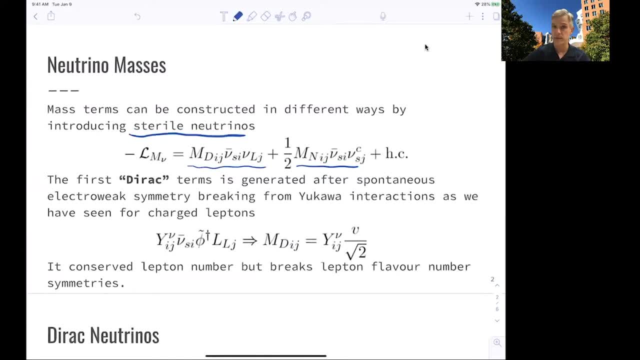 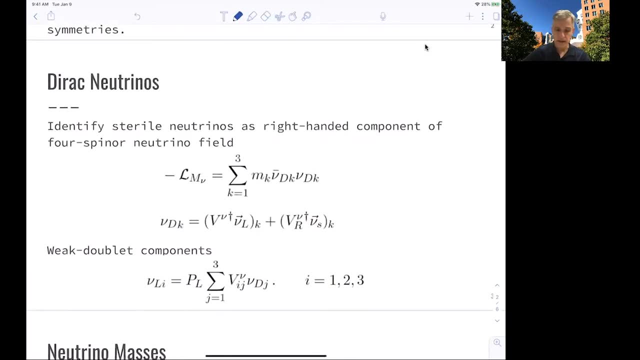 we have the same number of leptons but the lepton flavor is not conserved in this interaction. So we can rewrite this. So we identify the sterile neutrino as the right-handed component of the spinor. I mentioned this already And you know we basically couple the weak duplet components, as we would just expect. 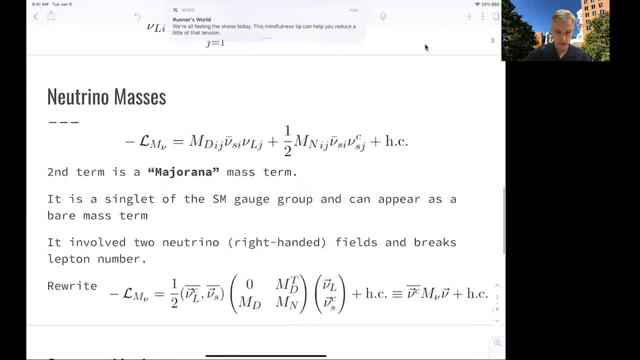 that to appear. The second term, the Majorana mass term, is interesting, as we introduce another singlet into the standard model. This then can appear as a bare mass term, with some consequences. So here, what we are trying to do is we're involved. 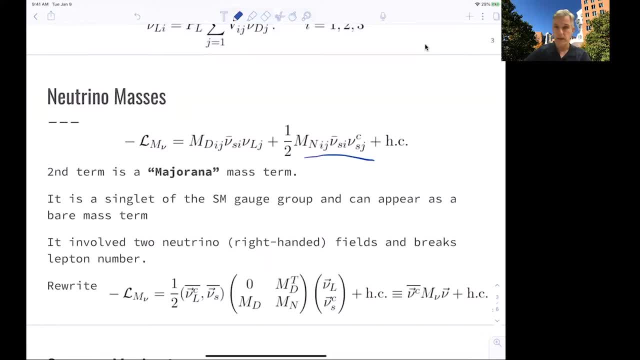 two neutrinos, right-handed fields, Those break the lepton number. So if those neutrinos are realized in nature, we have to observe lepton, We should observe lepton number-violating processes, And so the search for the specific kind of neutrino. 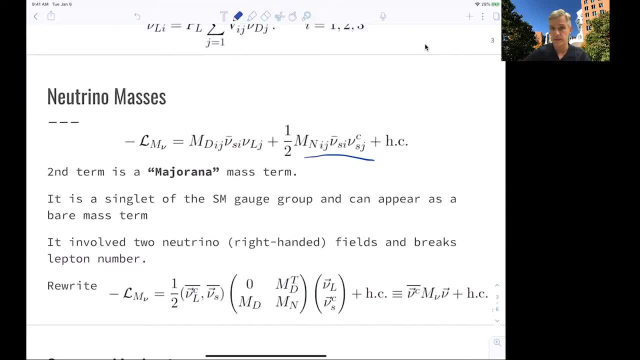 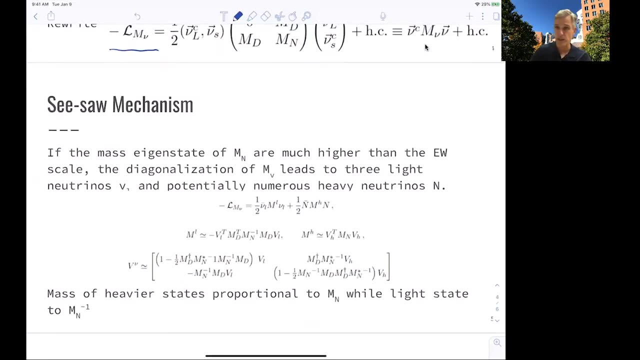 is through searching for lepton number-violating processes. So we can rewrite this part of the Lagrangian, this part of the mass term here, using this matrix. So let's see how this unfolds If the mass term now is much, much larger. 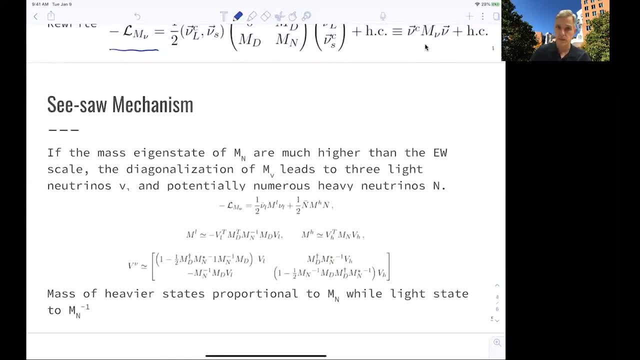 than the electroweak scale. you can try to diagonalize the mass term And it leads to three neutrinos, three light neutrinos- three neutrinos, you would expect, And one potential, or maybe multiple potential, heavy neutrinos. If you then rewrite the mass term, 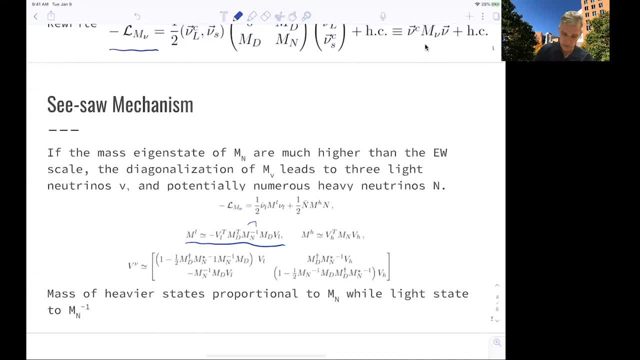 you find. for the light ones, the term which goes is one over the scale of this neutrino. That is a nice motivation for this kind of physics, as it automatically reduces the mass of the neutrino as we observe their masses to be very small in nature. 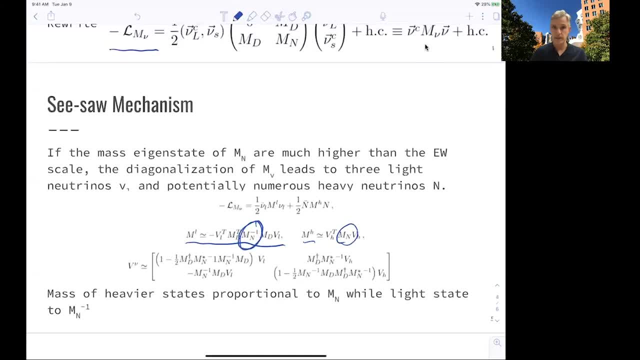 And then the mass. The heavy neutrino is proportional to the mass. This mechanism is called seesaw, because you automatically move the scales of those two neutrinos, the heavy ones and the light one, apart. So you have to observe the heavy one, maybe because they're 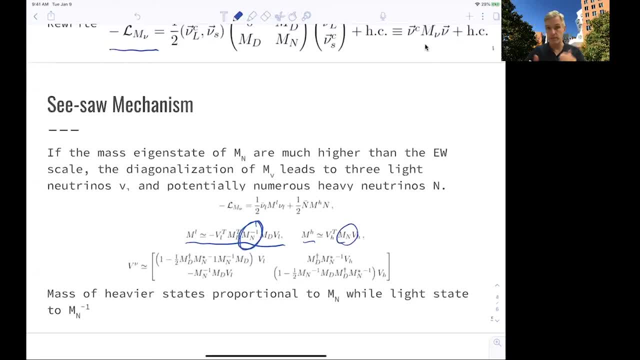 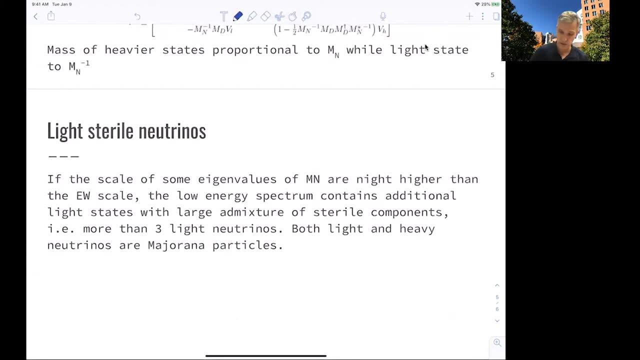 very, very heavy And the light ones have light mass because of this mechanism of being proportional to one over the mass scale, the mass eigenstate of those neutrinos. However, if the mass scale of those eigenvalues is much not higher than the electroweak scale, 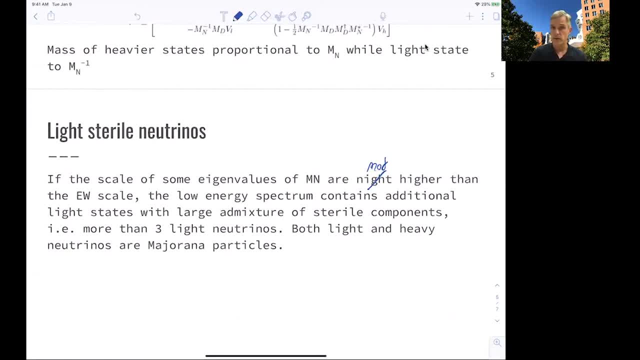 the lower energy spectrum contains this additional light states. So you have not just the three light neutrinos but you have additional light scales, states which mix with these three light neutrinos, And that is kind of an interesting area to look for these particles, as they would lead to say: 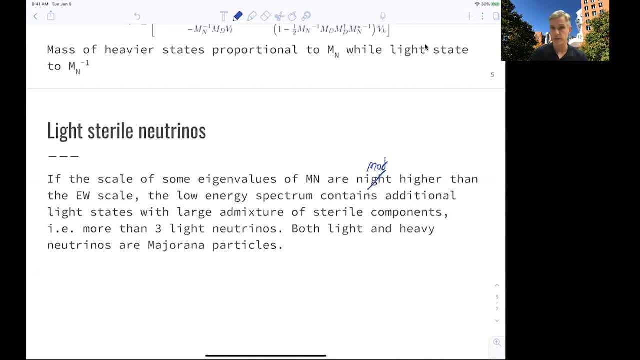 small deviations in observed electroweak position properties And they might yield to some interesting decays in nuclear physics And we'll come to those specifics later. But we have seen in this lecture two different ways to generate masses. One is to recover interactions same as the interaction. 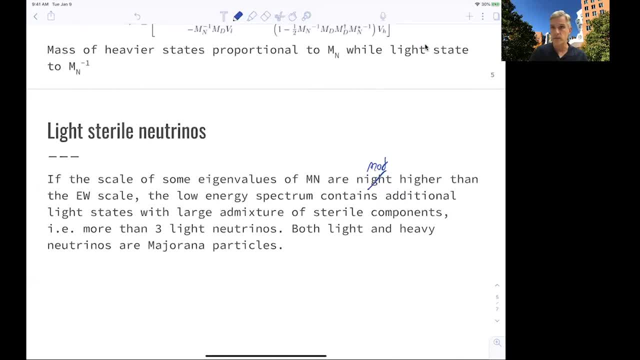 with the Higgs field And one we have, the seesaw mechanism, introducing Majorana neutrinos. This is a type of